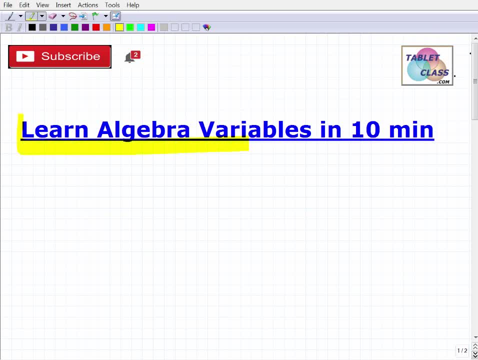 Okay, let's learn algebra variables in 10 minutes. So really this video might go a little bit shorter than 10 minutes, might go a little bit longer, but more or less I think we can cover a lot of ground in 10 minutes or so. 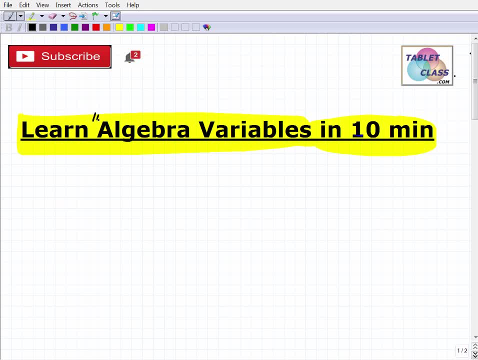 Now the title of this video could be a little misleading. It says: learn algebra variables. Really, it's just variables, and variables are part of algebra. So we're going to highlight some really important things about it and distinguish this idea of algebra. what makes it unique? 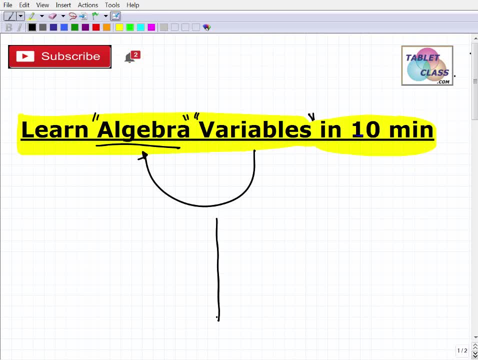 So let's take a look at something here real quick. So when you're first learning math, you're in elementary school, kindergarten, first grade, etc. You are doing things like 2 plus 7.. You're working with numbers, right, And this type of math here is basically what we call arithmetic, right? 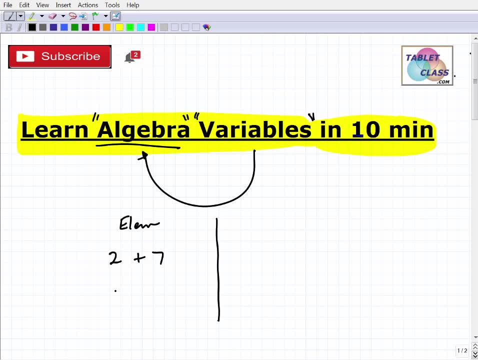 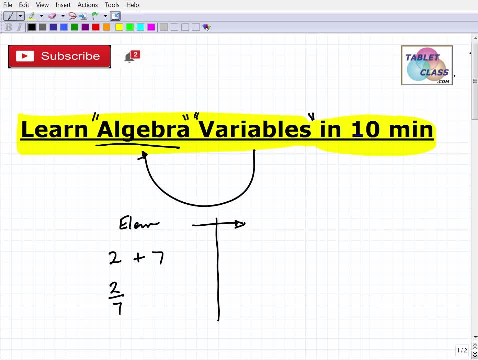 transition into your middle school years, especially your high school years, you're going to be learning algebra. okay, now, algebra, in a lot of ways, is essentially arithmetic. we're still doing, we're still working with numbers, but instead of actual specific numbers, we also use variables. so here we have, we're adding. 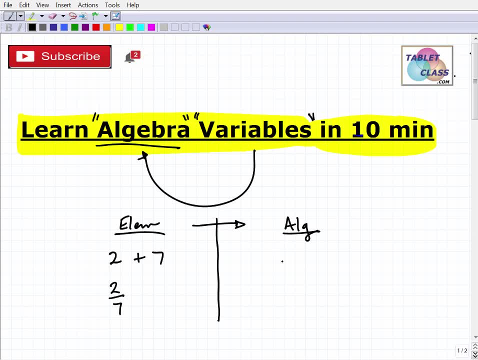 up two numbers, specifically 2 plus 7, but an algebra. we can have something like this: X plus Y, and this means that we're adding up two different numbers as well. so let me go ahead and define what a variable is, and then we'll go from there. 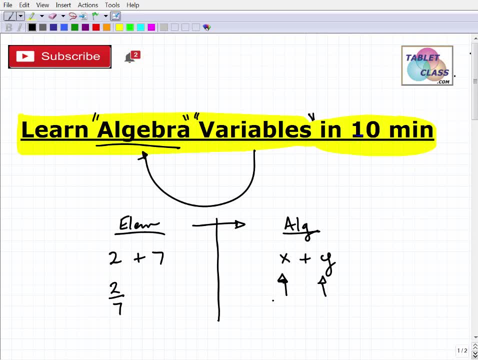 so a variable in algebra and mathematics is nothing more than a symbol. okay, oftentimes it's a letter that represents a number. okay, so anytime you see a X, a Y, a Z, a W, anything like that, it's a letter, that is a variable and we're adding up two numbers. so a variable in. 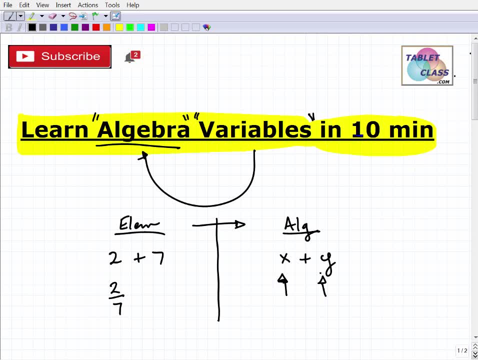 algebra in mathematics is nothing more than a symbol. okay, oftentimes it's a placeholder for number. now, what number do you want? or what number specifically does these variables represent? well, it's all up to you, okay. so, for example, I could say: well, let's just let X equal to 2 and Y equal to 7, so we can think of. 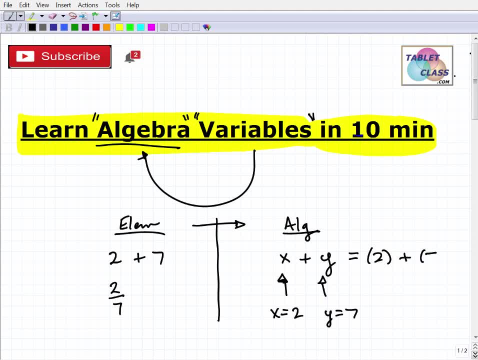 this expression as 2 plus 7, or I can switch this around and be like: well, it's X equals 1 and Y equals 9, and we can have another different problem: that we're adding up two different numbers. so in algebra variables are placeholders for numbers. now you've been actually working with variables for some time, you. 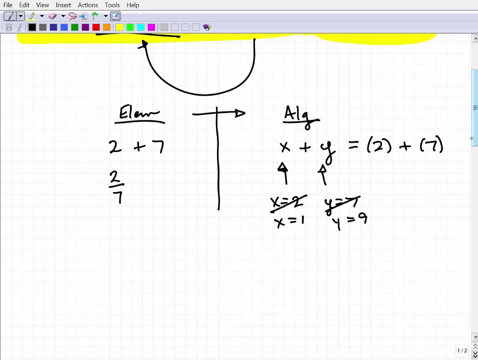 probably don't even realize it. so let's go back when you're like in first second grade. yeah, let's look at these problems right. remember your homework. I'm sure we all had it, even myself, I don't know. maybe it's probably been 有 four. 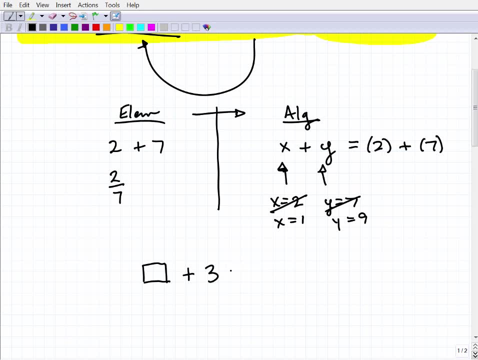 40 something years, kind of giving my wage here. But let's say I had a problem like this, right? Everyone kind of remembers this from first grade. So we have a box plus three equals five, And and you basically, hey, you know, to get the smiley face from your teacher, you have to figure out what number goes into the box, right? So this box is a symbol, right, It's not a letter, It's a symbol, but it represents a number, some number. we got a. 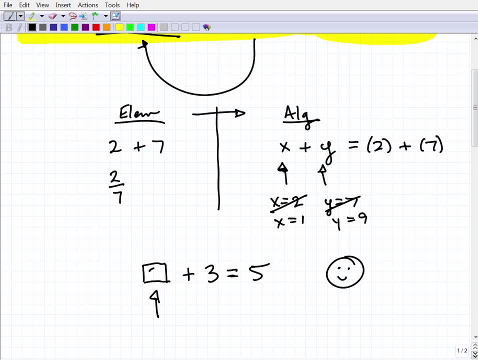 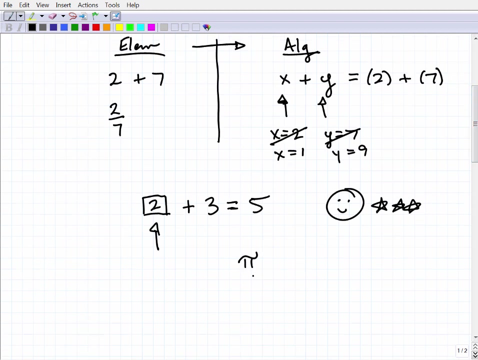 figure out what number to plug in there to make this true. Of course, we would all get. we'd all put two, we'd get all these little awards, a bunch of stars, etc. But this is the idea. So even at an early age, we have this concept of what a variable is. it's a placeholder for a number. Now, some other type of variables that you might be familiar with is something like this: So this is the symbol for pi. Okay, now pi, and hopefully most of you are. 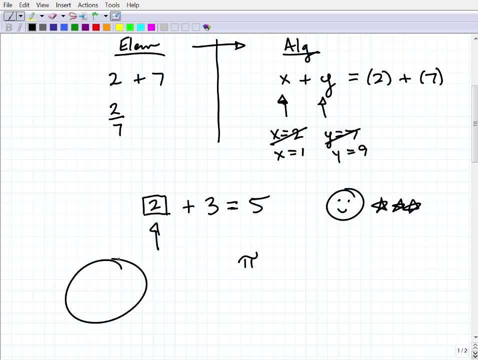 familiar with this. I'll just tell you very briefly: if we have a circle, if we take the distance around the circle- that's called the circumference- and we divide it by the diameter for any circle, you're going to get this number around 3.14.. And it keeps going on, and on, and on. Okay, this number goes on to infinity because the decimal part of this 3.14, it doesn't end. it's what we call non terminating and non repeating. So to know what 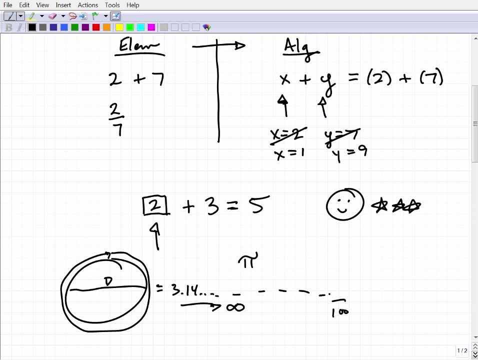 the digit. the hundredth digit is way out here. we'd actually have to calculate it out. So we won't. we'll really know, we really will not know what the end of this number is. So we say, you know what? we're not going to be, you know, crazy and write out this entire number, because you cannot write it out right. So we'll just say, listen this whole number, let's just assign it a symbol And we'll call it that pi. And then there's other famous ones in mathematics: a small e as you progress in your mathematics journey. 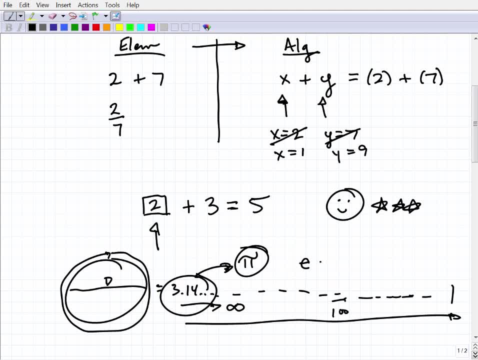 This is a very important number as well. It's approximately 2.718, if I'm not mistaken. on and on and on, And that has a big meaning in math. of course, pi is approximately 3.14.. So these are symbols, letters, you know, boxes, circles, even something like this: blank plus seven equals eight. this little underline we could consider a variable. it's a symbol, it's a placeholder for number. So let's talk about 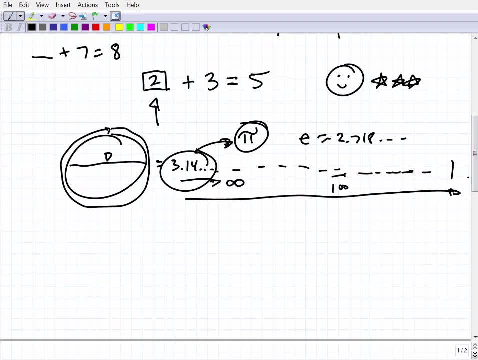 a few things here in algebra that you're going to see that are going to be relevant. So if I have x plus z, I have two different numbers. Generally speaking, I can interpret this. this is an algebraic or variable expression. we can kind of think of this as one number plus another number. So we have one number plus another number. 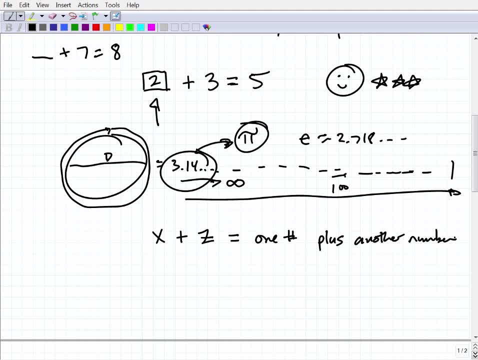 number. Now, the value of z and x can't be the same, but this is a good phrase to represent what's going on here: x plus y, one number plus another number. You're going to have to know how to do this when you're working with. 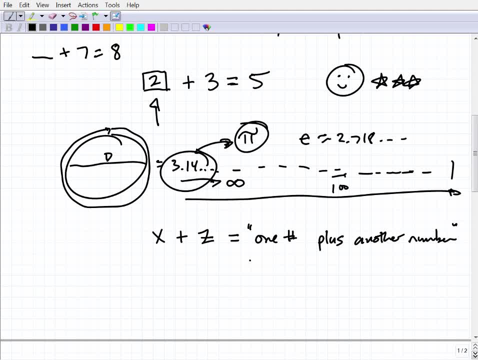 variables. You're going to have to be able to take a verbal statement and translate it into a variable statement. So this is part of a set of skills that you'll need to learn as you progress in your math journey. Now let's take a look at something like this: 3x. So if I write the number or a number in 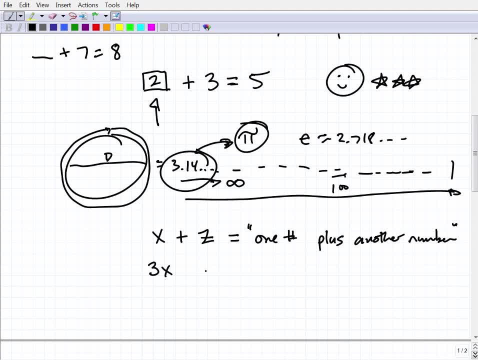 front of a variable. let's say, for example, 3x or maybe 8y or negative 10z. What does that mean? What does this three in front of the x mean? here Doesn't mean three plus x. this is that would be this: 3 plus X. it's certainly not 3 minus X. this is. 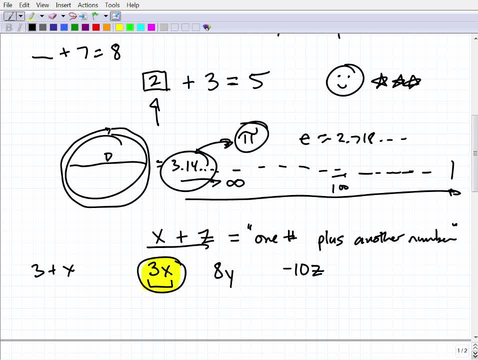 multiplication. okay, this means 3. X is 3 times X. this is the product of 3 and X. so in algebra when you see things like this, the number in front of this variable is is a product. okay, so this is 8 times some number: Y. okay, this is. 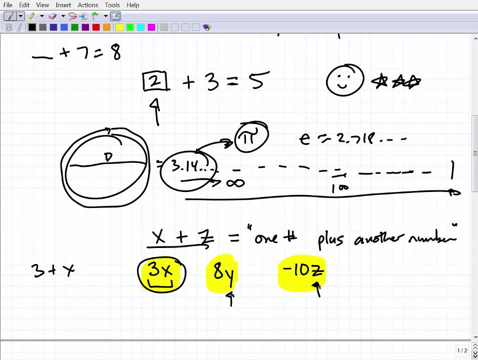 negative 10 times some number Z. so in algebra- kind of a little terminology, these little guys here are considered terms. this is a term, okay, and the number in front of the term is called a coefficient- coefficient- just kind of abbreviate that because I'm sure I'll misspell it. so we have a coefficient and 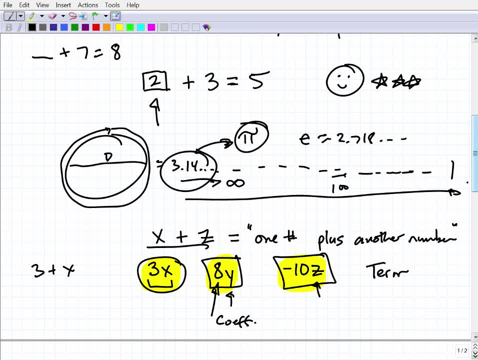 we have a variable, and then sometimes too well, I even have powers. let me go ahead and show you how that looks. so let's say, we can have 3 X and 3 X squared. so this is one term. okay, the coefficient is 3, the variable part is X, and then this is a another term: go ahead. 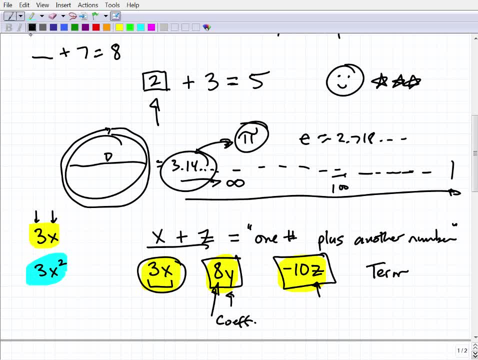 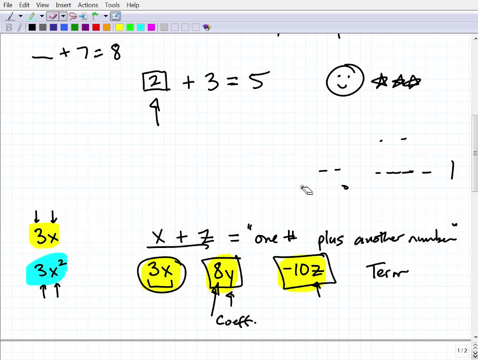 and highlight this. so the coefficient is 3, but the variable part here is X squared. now, something that you're going to have to definitely know about- and I think we'll kind of call it a wrap here after I could just kind of introduce you to this concept- is the concept of like terms. so, like terms, okay. 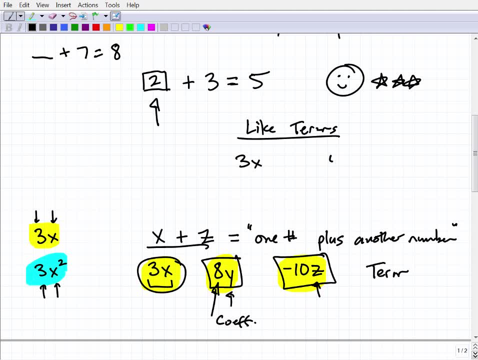 so let's say I have 3 X and 4 X. now these two terms here, these two terms we can, we? we consider these guys like okay, so let's think of them like terms, okay. so now, the reason why they're like- remember, these are independent terms- is because they have the same exact variable part. 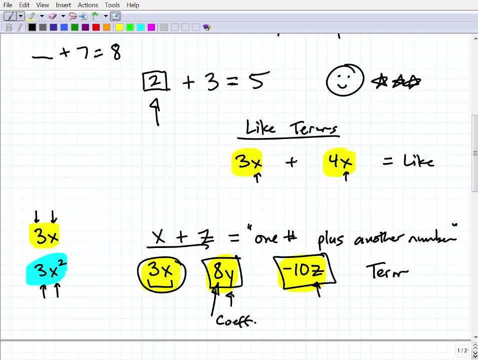 so in algebra we can actually add these guys or subtract them. so 3x plus 4x is equal to 7x. so in algebra when you have like terms, you can add them up by simply adding the coefficient parts. but let's take a look at another scenario. let's say I have 3x plus. 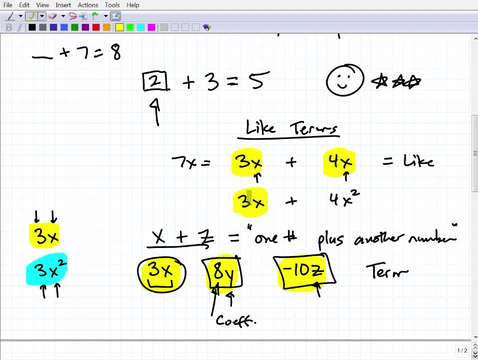 4x squared. okay, so I have one term here and I have another term here. now, in this case, this example, these are not like, not like terms. now, what do you think that is? hopefully, it's pretty obvious to you that this is an x and this is an x squared. so the rule is: 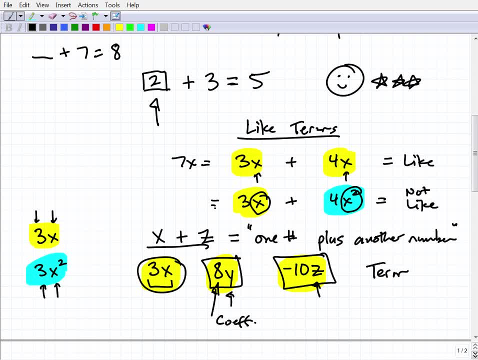 if the variable parts are different, you cannot add them. okay, we can't add these guys up, alright, so we just leave this expression the way it is. that's as simple as it can go. so 3x plus 4x squared is as simple as we can write that in algebra. however, 3x plus 4x, we want to write that: 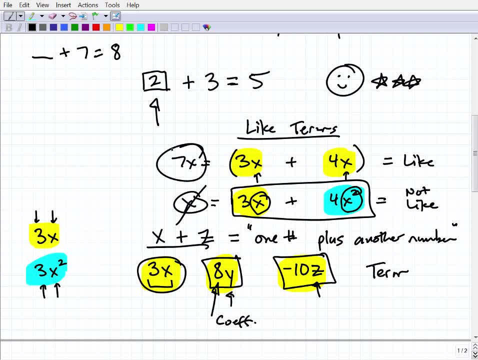 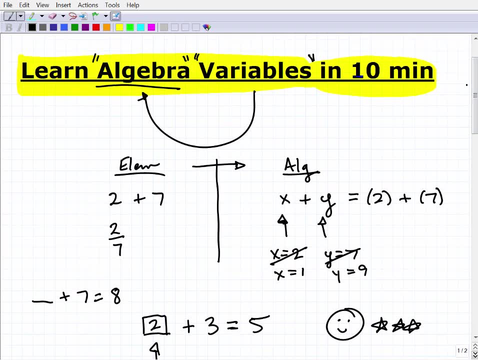 as 7x. okay, alright, so I think I'm pretty close to the 10 minute mark and hopefully you know you definitely got- I think we covered- a pretty decent amount here, certainly about variables. of course there's a lot more to learn, but one you know, you know you should have. 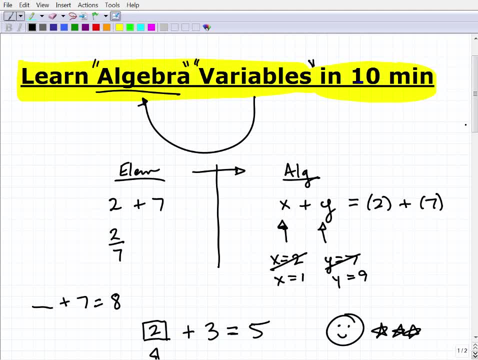 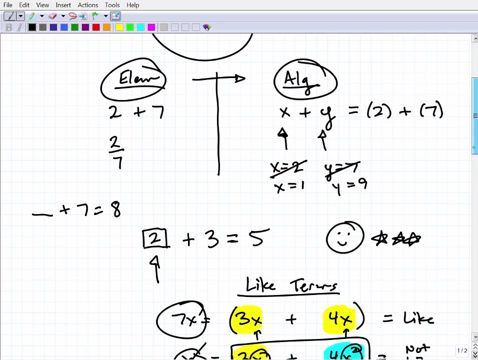 you know, we got a basic definition what a variable is. right, it's a placeholder for number. we also distinguished why we kind of need them, because in algebra we start using variables okay, and that's different than what we've been doing in elementary school. and then we talked about terms. 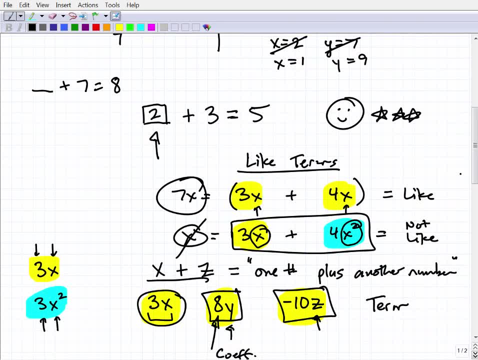 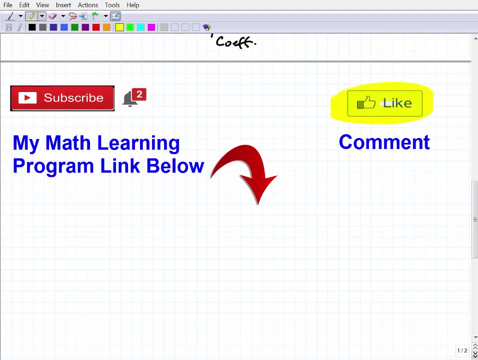 what they are and like terms, et cetera. okay, so, so I'm going to wrap this up. if you got something out of this video, I certainly hope you would consider giving it a thumbs up, and also, I literally have hundreds of videos on my YouTube channel, of course, if you haven't.